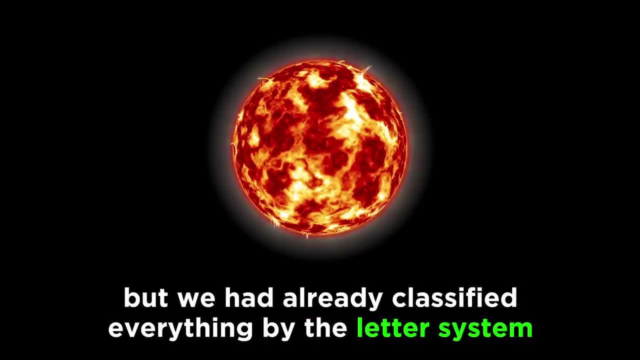 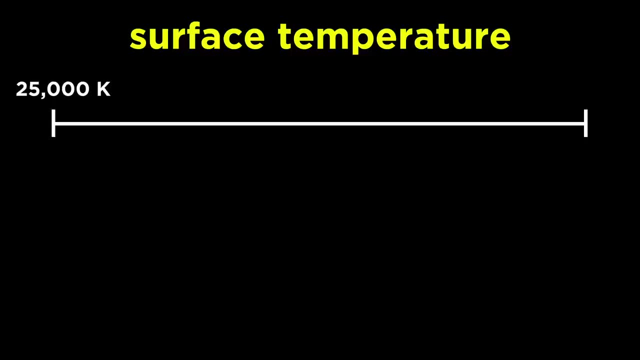 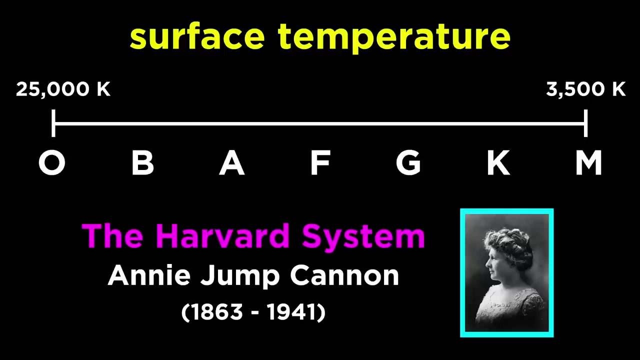 categorized by surface temperature. But this letter system was retained because all the work to classify stars had already been done. So, from hottest at around 25,000 Kelvin, to coolest at around 3,500 Kelvin, we now have O, B, A, F, G, K and M stars, a classification system called the Harvard system, which was 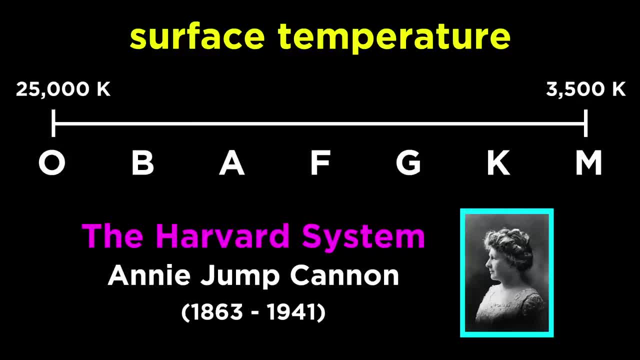 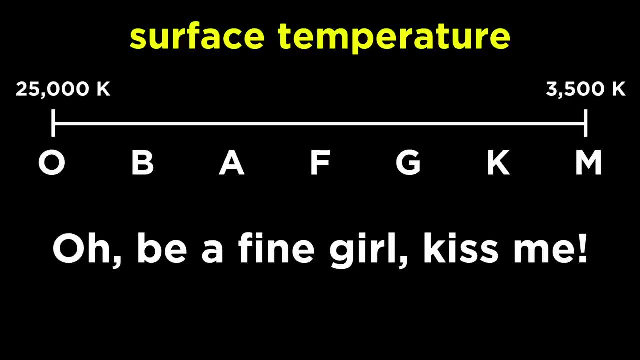 developed by early astronomer Annie Jump Cannon. This system is called the Harvard system. This sequence of letters is rather unintuitive, but to remember the order we can use the following mnemonic: Oh, be a fine girl, kiss me. Feel free to replace girl with guy, depending on your persuasion. 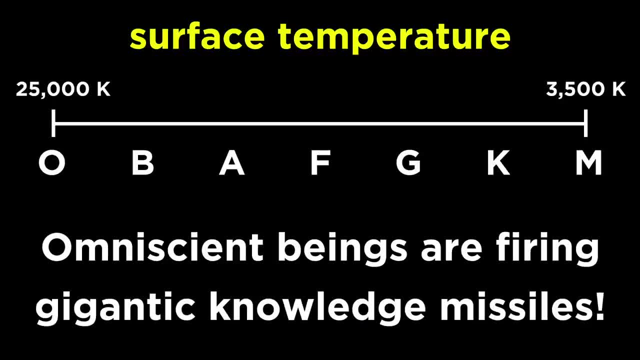 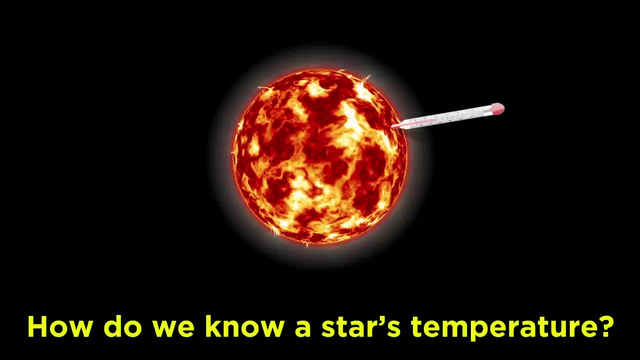 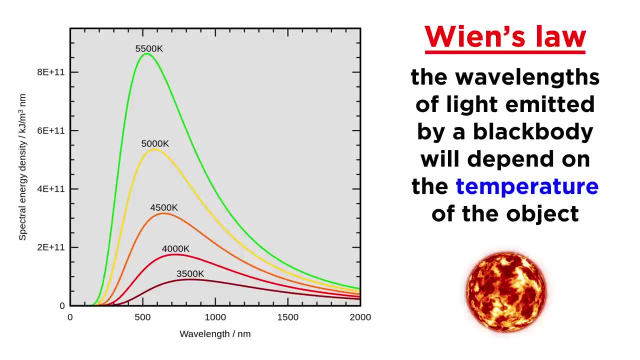 Or if you find the whole thing terribly sexist, just make up your own, such as: omniscient beings are firing gigantic knowledge missiles, As we can't stick a thermometer into a star to see how hot it is. this classification based on temperature is actually derived from Wien's law regarding black-body radiation. 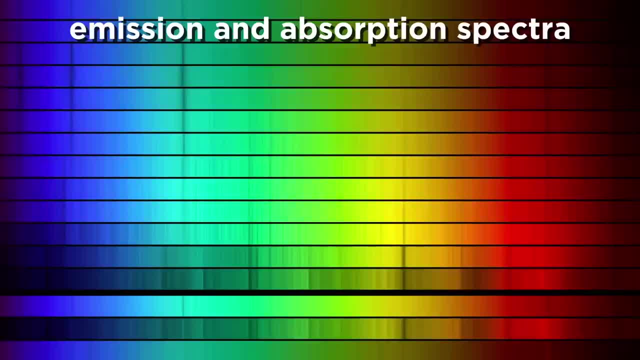 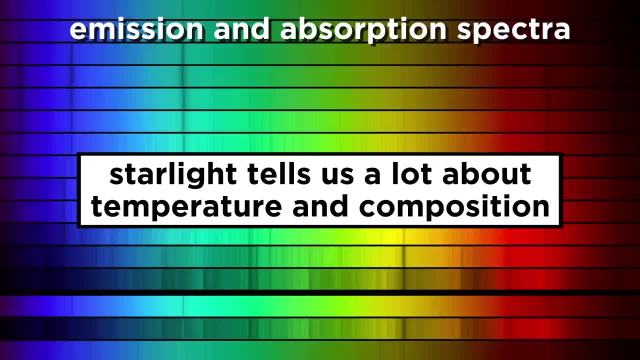 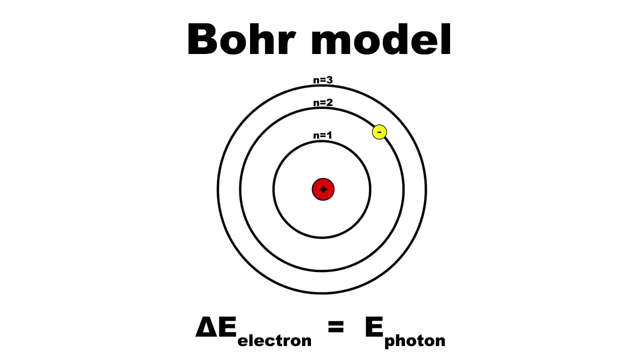 which we saw in the modern physics series, as well as other types of data like emission spectra. We analyze the light we receive from a star and correlate it with a particular temperature as well as with specific elements, just like when we learned about the Bohr model in general. 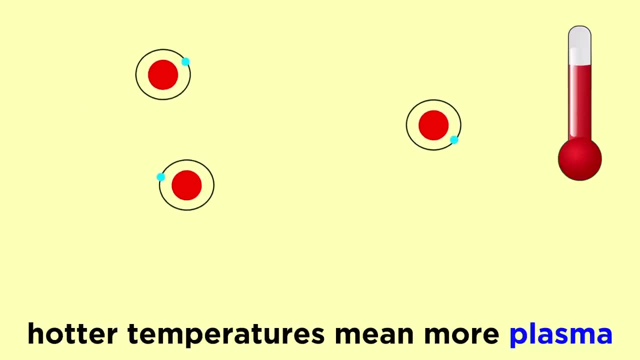 chemistry, The hotter the star, the more of the hydrogen and helium nuclei are released into the star, and the more of the hydrogen and helium nuclei are released into the star, We can use the idea that the helium nuclei are free to rotate and go out into space to 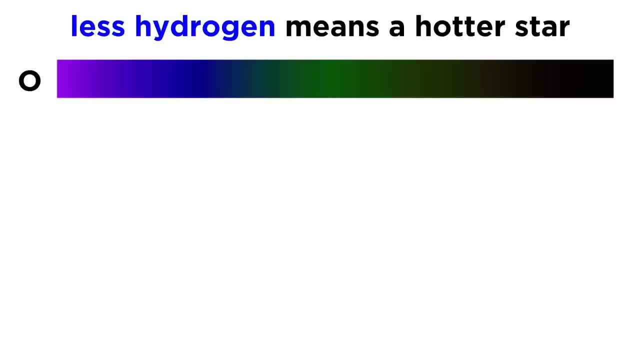 capture some of the burnt down elements, for example the gamma and gamma rays that have been stripped of their electrons, forming the phase of matter known as plasma. The hottest stars- O stars- show very little hydrogen, because most of the hydrogen is. 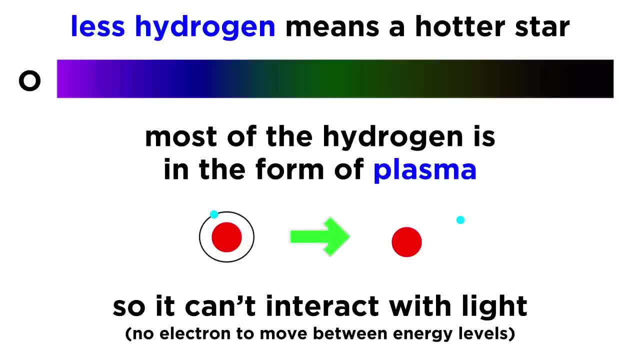 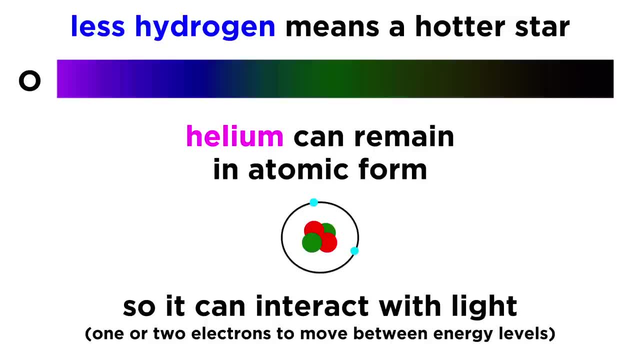 without an electron and thus can't absorb and emit light. Helium is still able to retain one or both electrons, and thus we do see emission correlating with helium Cooling down a little with A stars. suddenly hydrogen can hold on to an electron very. 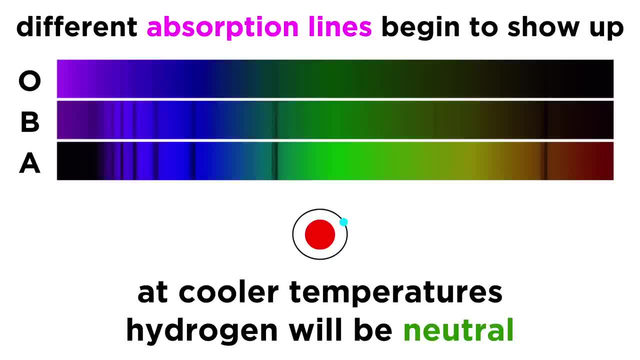 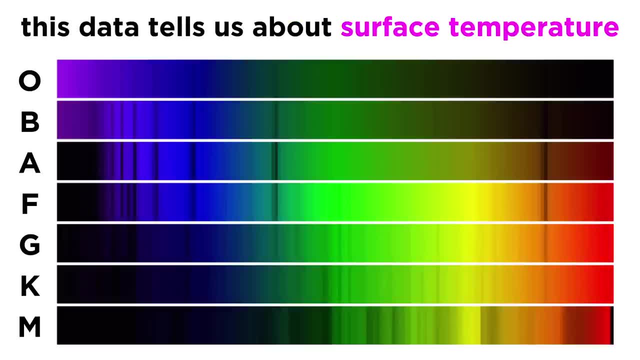 easily. It's because the light is in general a more difficult requirement of the free energy of an electron, so the spectrum changes, Getting cooler still. some bands show up that correspond with metals like calcium, So the convention is derived from temperature, but this happens to correlate with color and 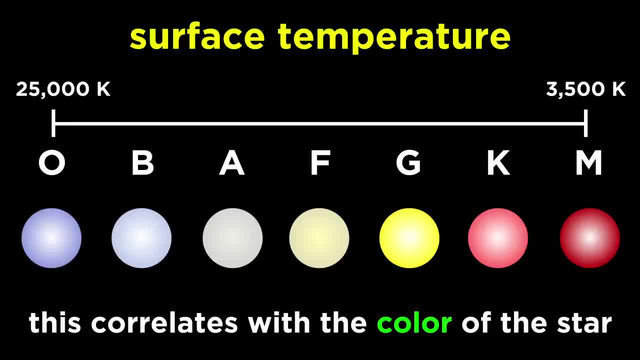 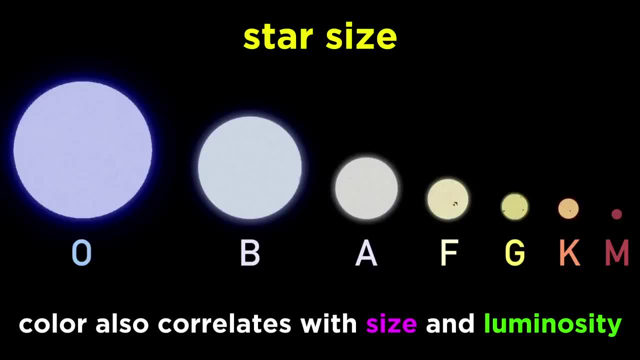 size as well. Hotter objects like O and B stars are blue, and cooler objects like K and M stars are red. Also, hotter stars tend to be larger and burn brighter with the additional heat resulting from the fact that so much more fuel is being burned. 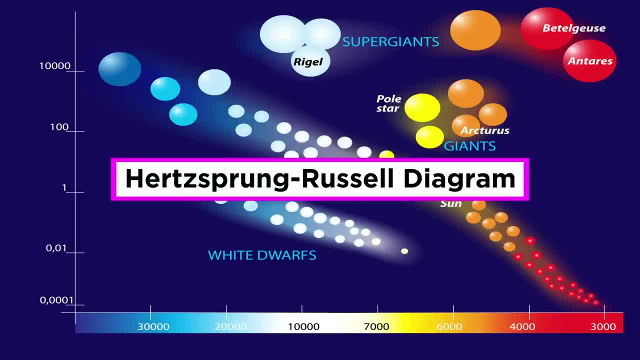 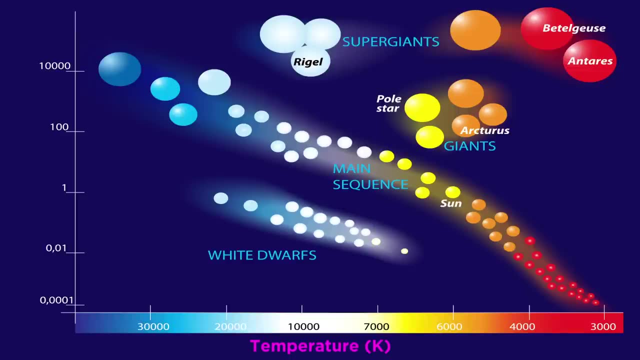 All of this- data regarding temperature and luminosity, as well as indirect information on mass and radius, can be represented on something called a Hertzsprung-Russell diagram, or an HR diagram, for short. In this diagram, the horizontal axis shows temperature decreasing to the right and the 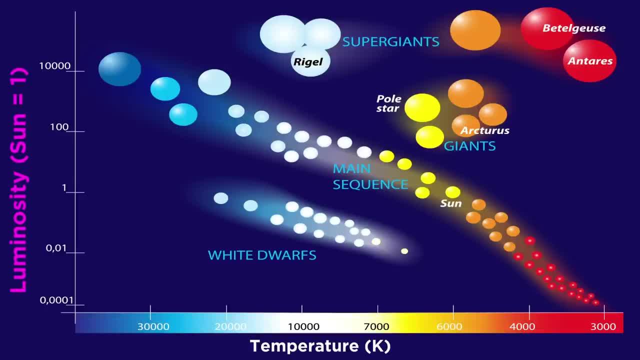 vertical axis shows luminosity or the amount of energy emitted by a particular energy. In this diagram, the horizontal axis shows the amount of energy emitted by a particular star per unit time increasing going up. We can see that the majority of stars fall on a continuous curve, which we call main-sequence. 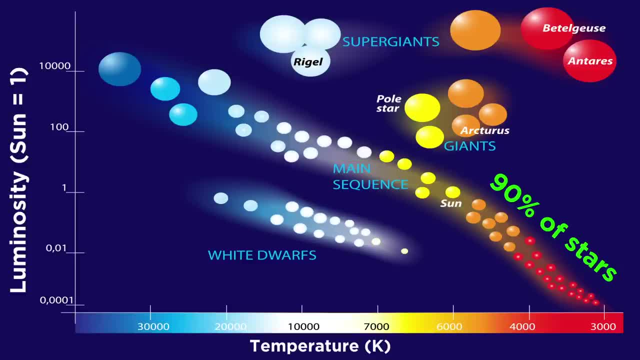 stars. 90% of all stars- follow this trend, including our own sun, which is part of this yellow region. here, Some stars, like red giants, are very cool yet luminous, while others, like white dwarfs, are very hot yet dim. 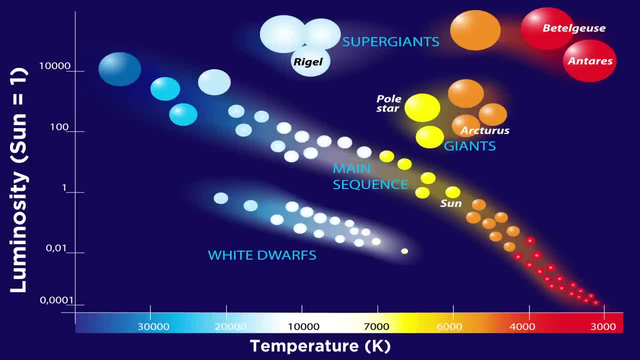 But the majority belong to this main sequence. Even though this diagram lists only temperature and luminosity, we can infer many things about other variables. Larger stars are always more luminous as more surface area means more energy emitted. We can also see color clearly correlating with temperature as we move from left to right. 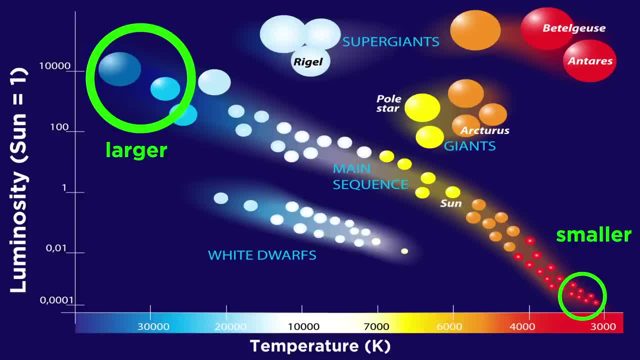 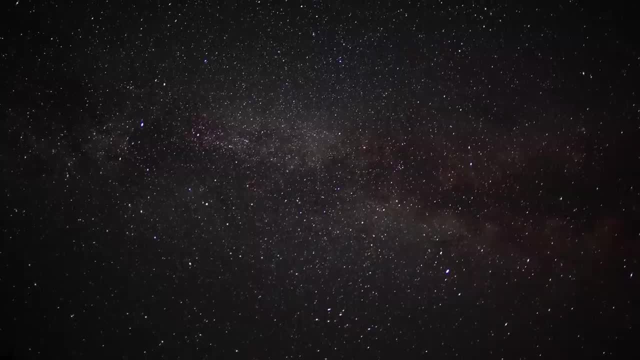 Size is also represented, with main-sequence stars decreasing in size from left to right, but with red giants and white dwarfs deviating from this trend. This data collected by looking at hundreds of thousands of stars in the early 20th century. 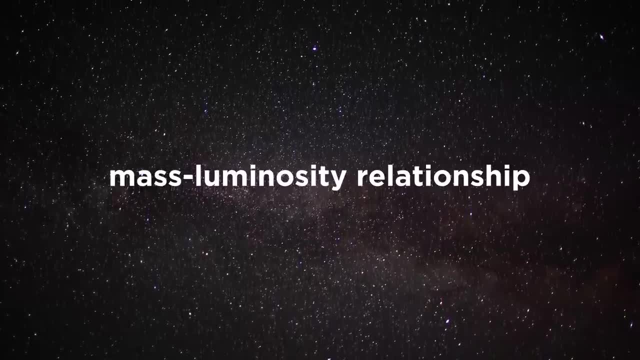 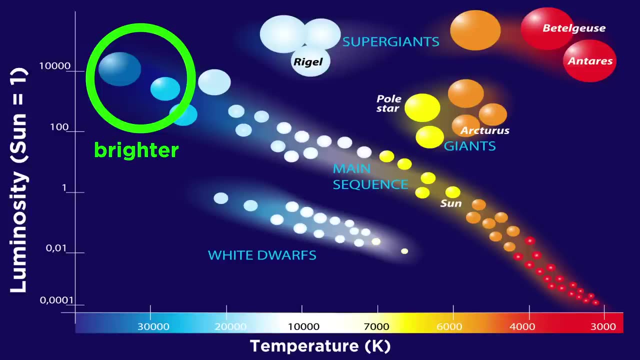 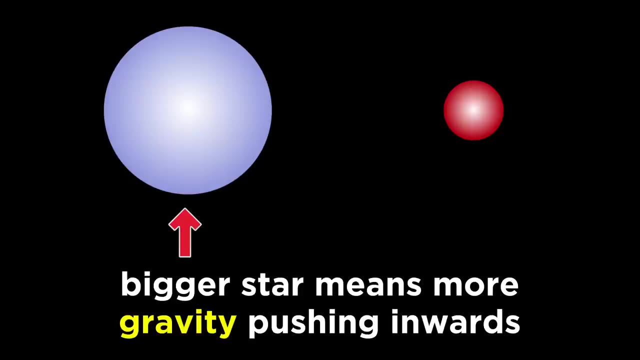 reveals certain facts about stars, such as the mass-luminosity relationship that we just described. It explains why the blue stars in this corner of the main sequence burn brightest, getting dimmer as we go towards the smaller red stars. This has to do with the fact that the gravity crushing the star inwards increases exponentially.